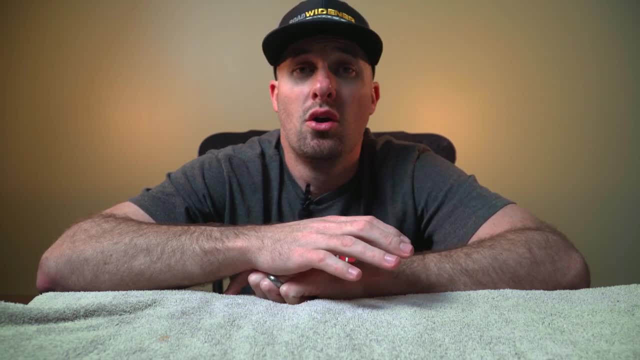 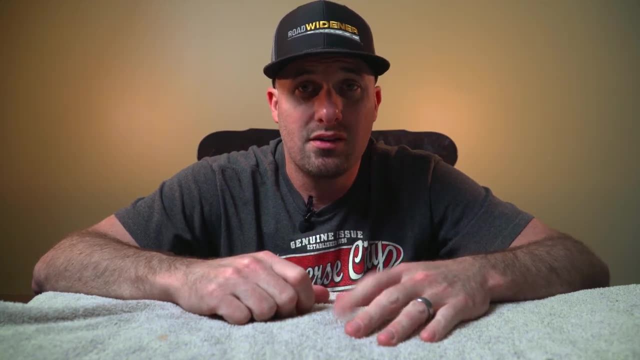 multi-directional flow. I mean they can get really complex quick. What we're going to cover is the fundamentals of how that system works and why it works the way that it does. I've actually got some tools today to help me out, So I've got my towel laid down here, because I've already 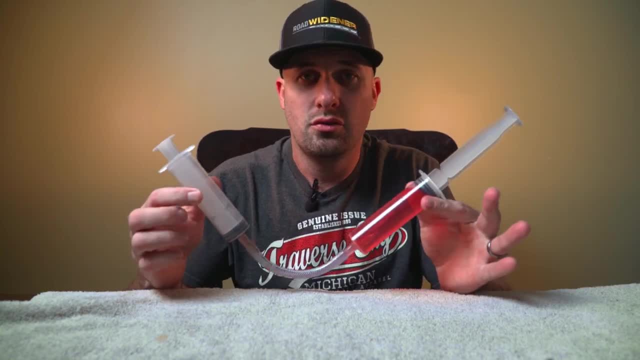 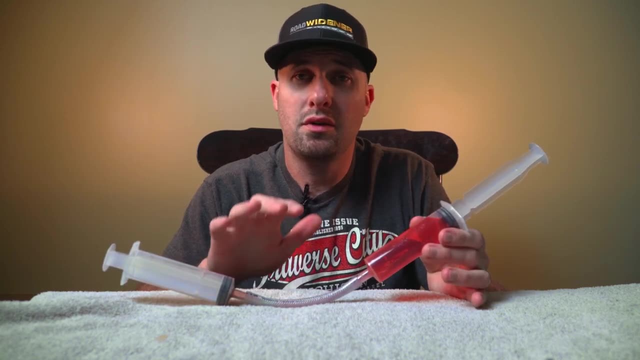 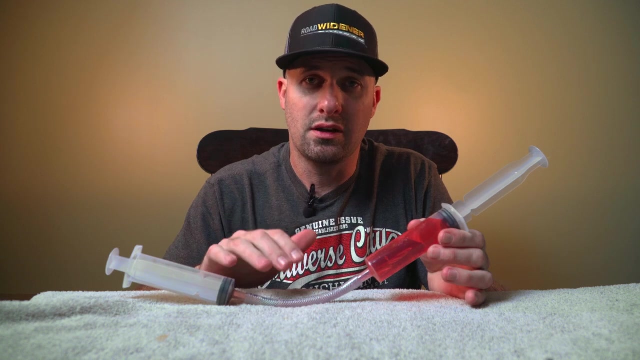 made a mess actually putting this whole thing together, But we're going to demonstrate a very basic hydraulic system. So first of all, the term hydraulics, you should know, does not refer to only hydraulic systems like we see on our machines. Hydraulics is really anything having to do with 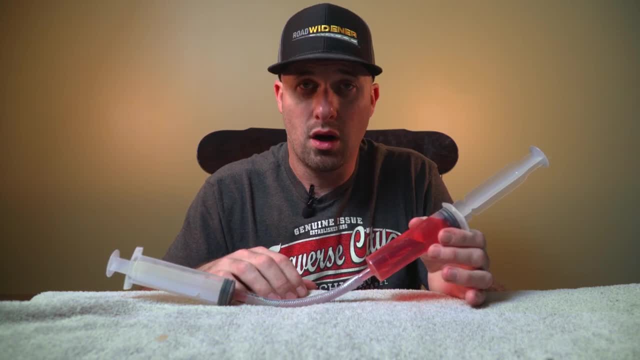 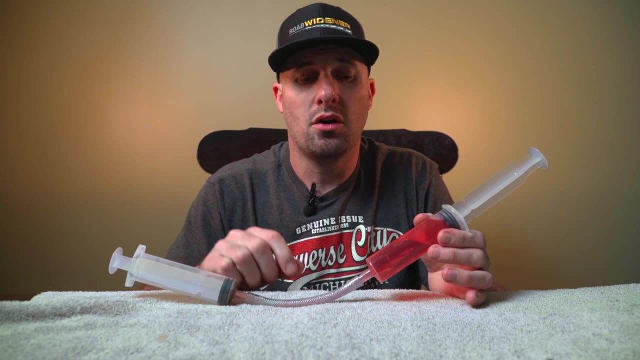 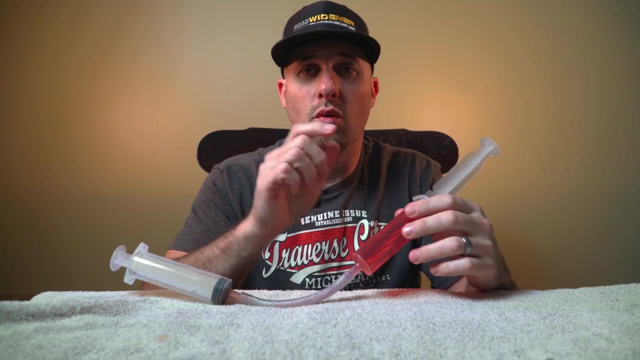 liquids. That's why, when you hear about guys talking about dams or water based structures, you will hear hydraulics thrown around. It's because it's it has anything to do with liquids and flows. It's about the flow of hydraulic oil through a machine and how it makes the machine work. We're 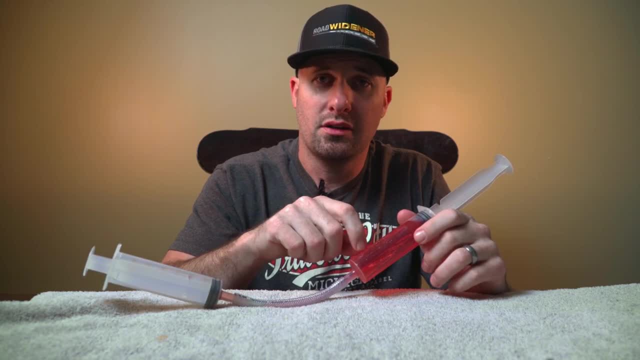 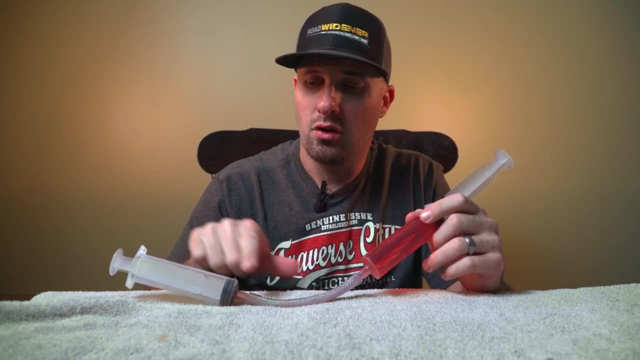 going to pretend that this side over here is our hydraulic reservoir and this plunger that I'm going to manually push is going to be our hydraulic pump. We have our hydraulic line going out to our hydraulic cylinder. So you know, I know this is another syringe, but let's pretend this is the rod. 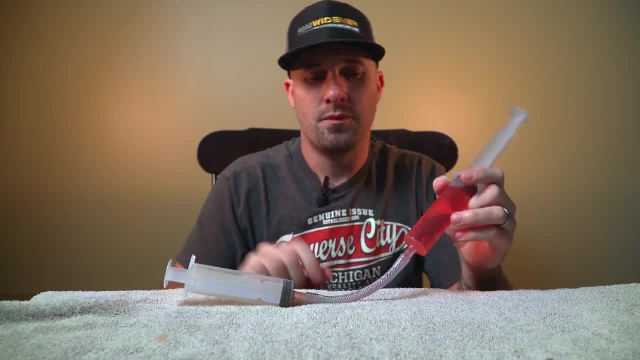 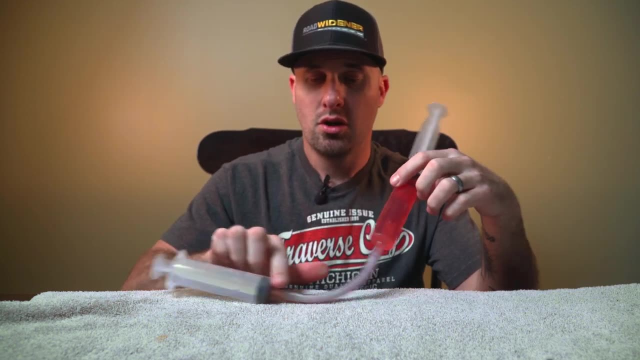 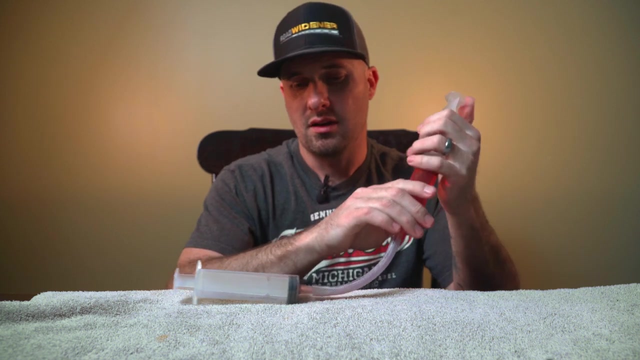 coming out at the end of the cylinder. This is the cylinder body itself. So what happens- and I know you already know what's going to happen, But when I apply a force and pump this liquid through my hydraulic line, the hydraulic oil only has one place to go, and it's by pushing this plunger out. And sure enough, when I start to, 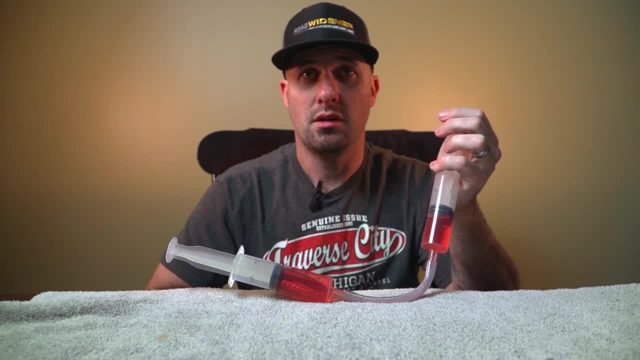 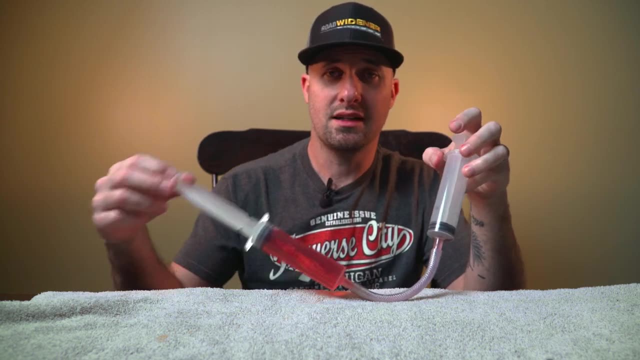 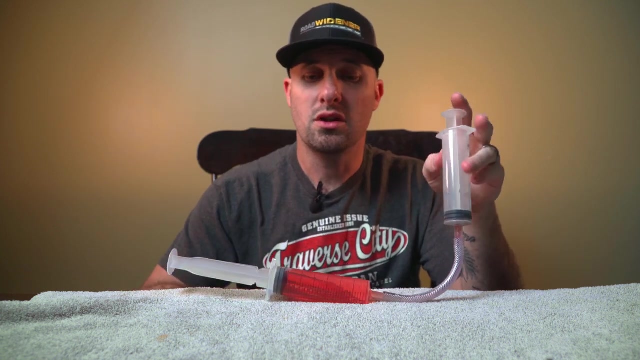 apply force. you see that plunger. we make sure in the camera. you can see it. good, that plunger moves out. Well, if you can imagine we had a bucket or something attached to this end, it's going to cause that bucket to move, It's going to cause the stick to move in and out. So that's the basics of what's. 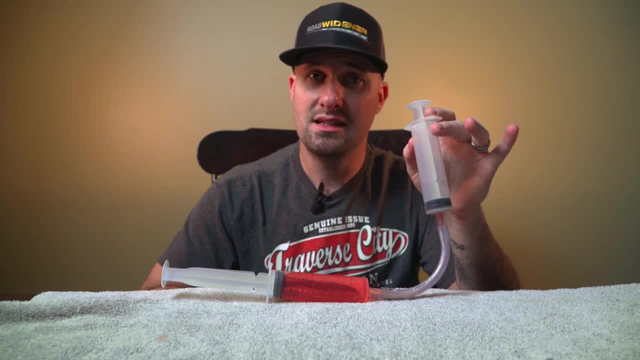 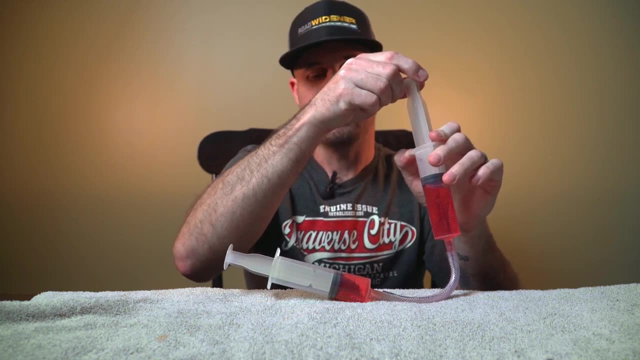 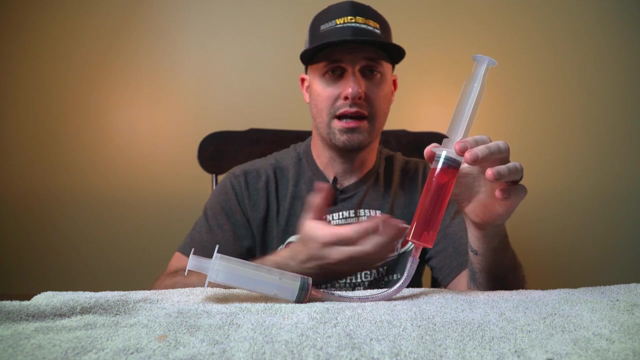 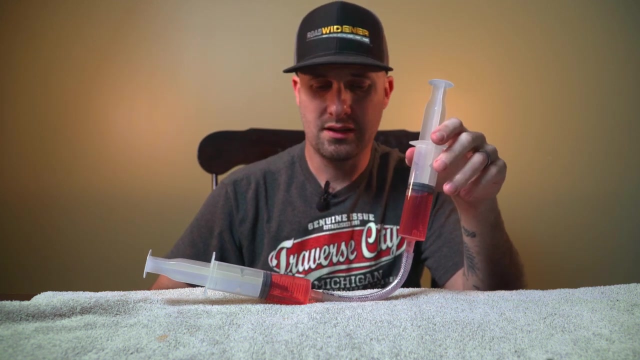 going on in this system. Now, where this differs is: in order for me to get this to retract, I actually have to suck the hydraulic oil back through the plunger. In a real hydraulic system, you don't suck hydraulic oil. What happens is: let me push the plunger halfway. What actually happens in a real hydraulic system? 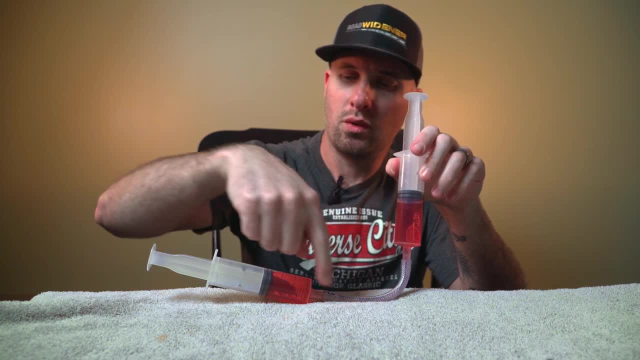 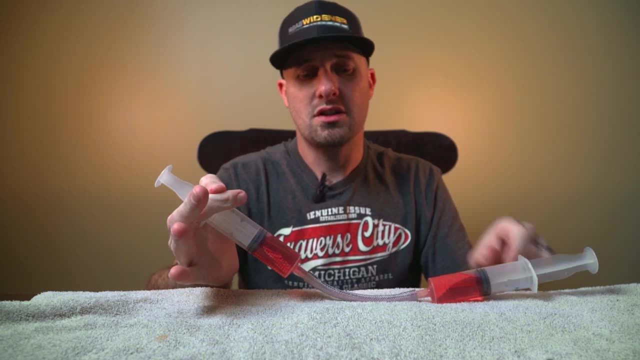 is. you can imagine there's a split here in the line and we had another line going up on this side of the plunger, And imagine that this was entirely closed off. Instead of sucking hydraulic oil back through your hydraulic line, what happens is the pump actually pumps on this. 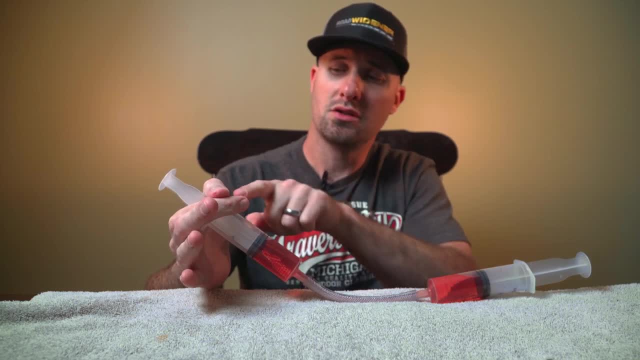 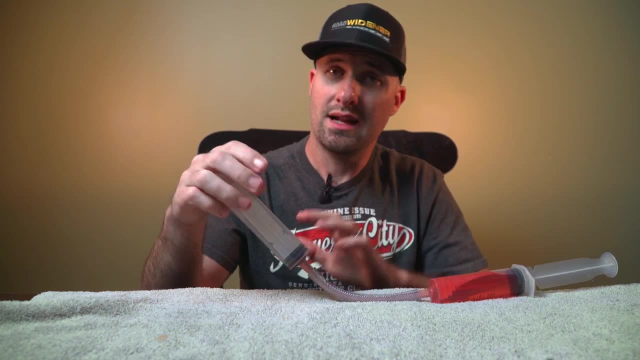 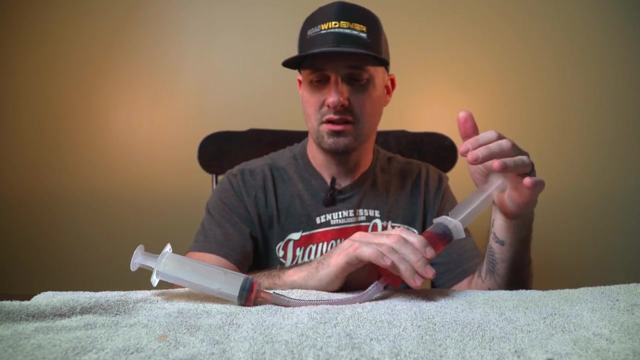 side of the plunger and it pushes the plunger back down, So you're actually forcing the rod to go back into the cylinder body. So that's the main difference between how a hydraulic system on an excavator works versus this little simple model here, But the effect is still the same. 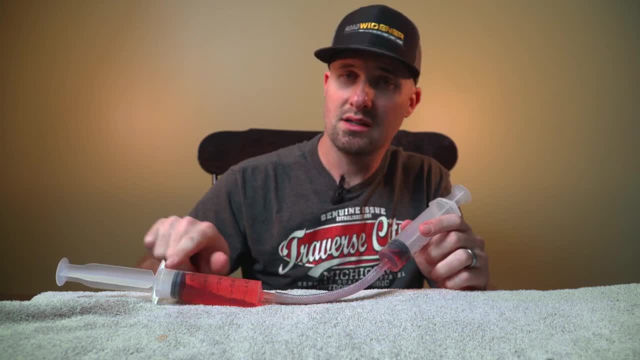 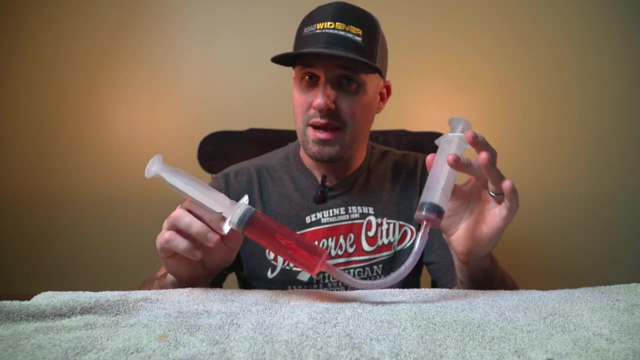 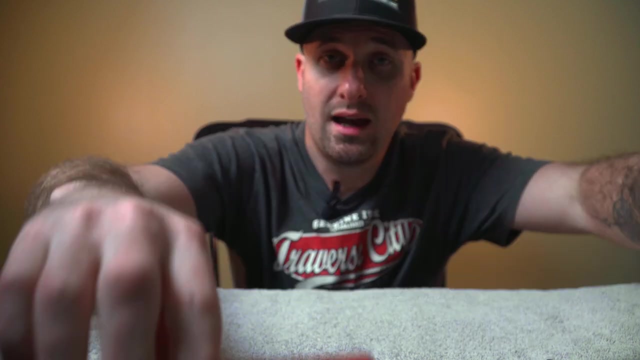 When we pump hydraulic oil through this line, it's going to cause the plunger to move out, and that will apply work to whatever we're trying to get done. So that's the basics of a very simple hydraulic system, But we get pretty complex on these machines, don't we? Well, I have a surprise. I have a more. 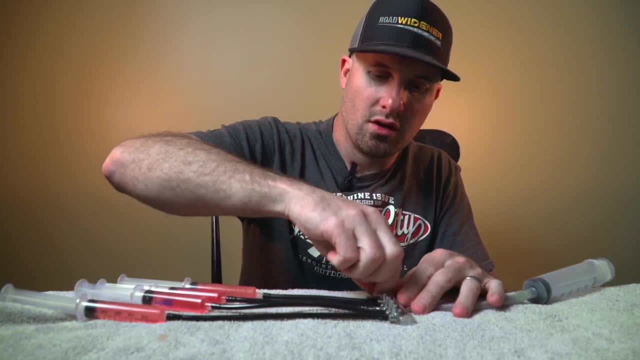 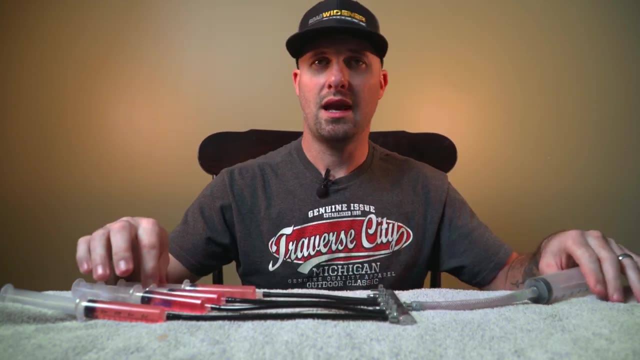 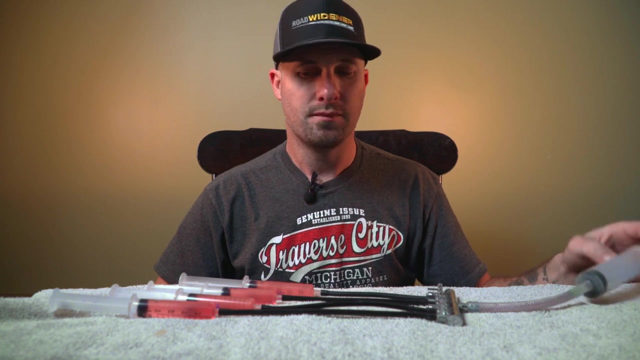 complex system. I know shocking, isn't it? So what we've got here is a series of valves that I can manually open and close, And we have it attached to- let me make sure everything's in focus here and in the picture- and we have four separate cylinders, So right now you can see that we've got liquid in all of. 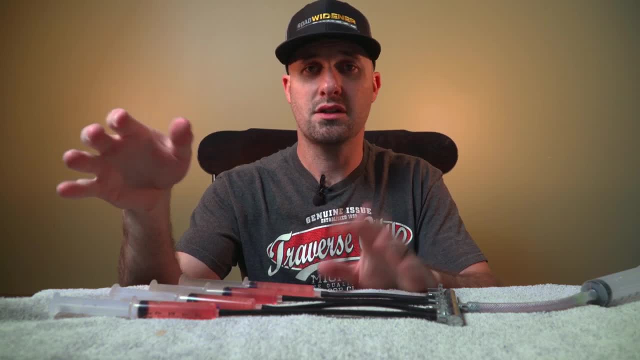 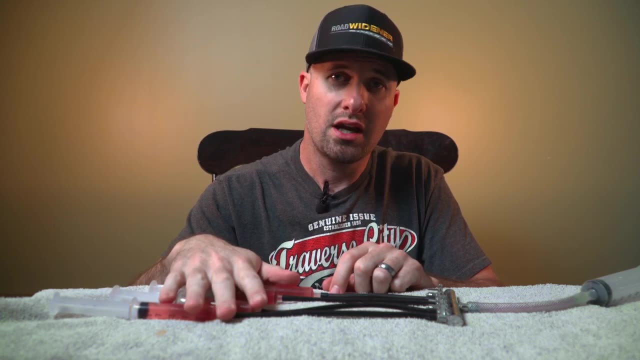 our cylinders out on the machine. And you may remember from my excavator tips and tricks which if you haven't watched that click up here on the link so that you can actually know what I'm talking about. But remember when I talked about checking the hydraulic oil level on an excavator. 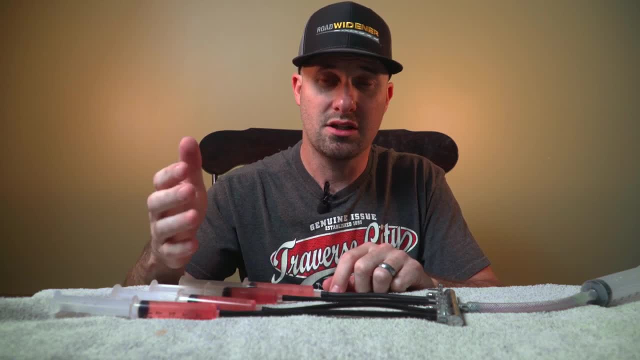 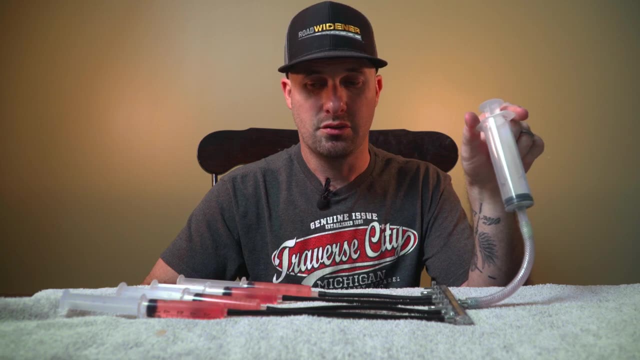 one of the most important things was making sure the machine was in the right position. This is why You can see that my hydraulic tank is totally empty of hydraulic oil in this situation, because the hydraulic oil is all out in the system. If we had a sticker in our machine that said, hey, you. 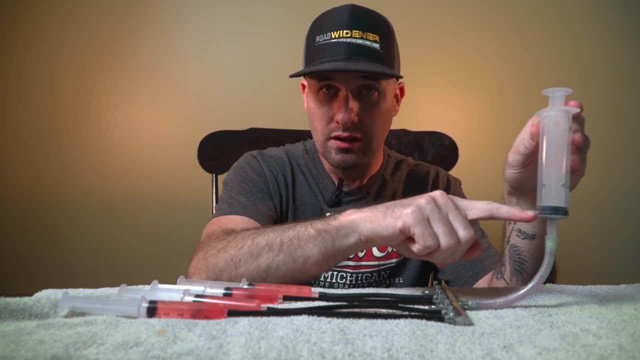 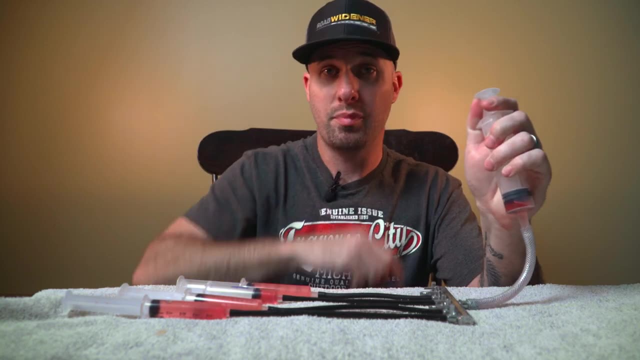 need to check it when all of your cylinders are extended and the hydraulic oil levels way down here on your tank. we're in good shape. Now what you're going to notice. I'm going to start pulling on this. I'm going to start pumping our hydraulic oil back into the machine. What's happening to? 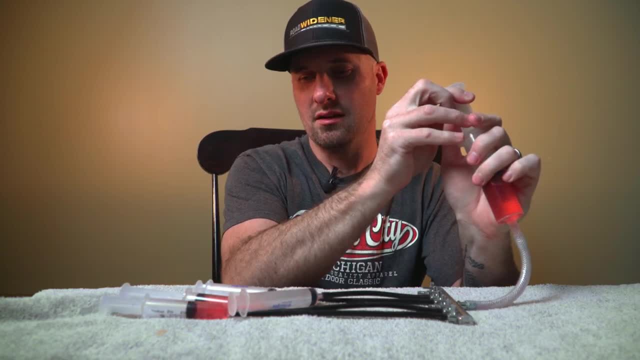 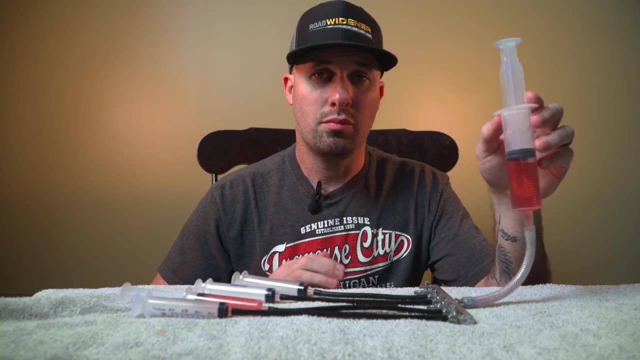 our plungers if you can see that they're all starting to suck in. So let's go with that position right there. This is probably a more realistic look at what it would be to check the hydraulic oil level on an excavator. So maybe we've got our stick cylinder. 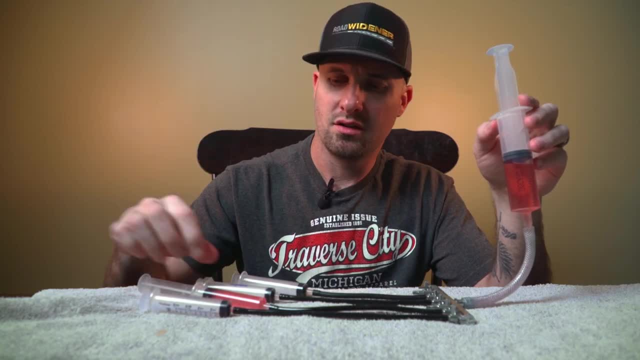 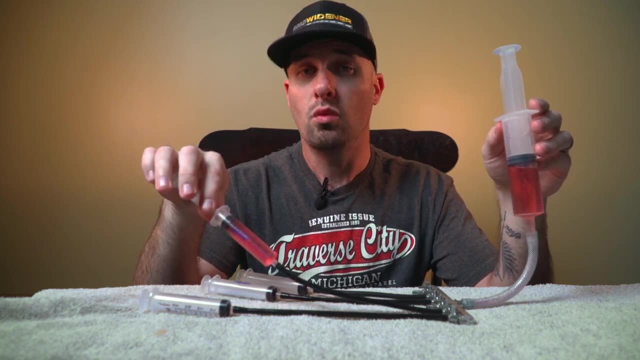 that's about halfway out like this, but all of our other cylinders are retracted, which means that we have accounted for this oil here not being in the hydraulic tank when we go and check our hydraulic oil level, And sure enough, we've got our sight glass, we've got hydraulic oil there, we're good to. 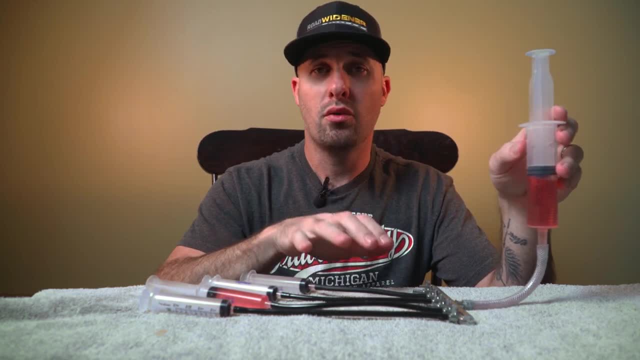 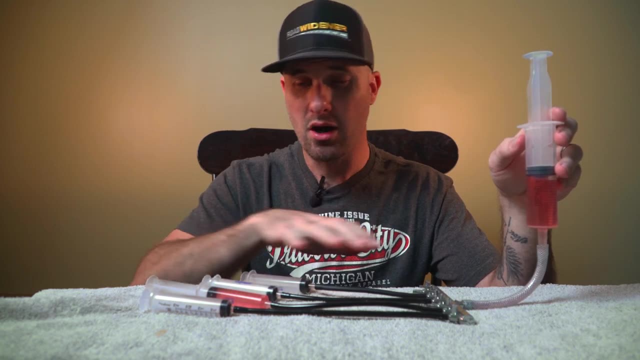 go for the day. So just a quick Side note. that's why it's important to make sure you check hydraulic oil levels when the machine is in the position that the manufacturer tells you it needs to be in, because they are accounting for this right here. So let's go back to our hydraulic system. So what we've done is we've made a very 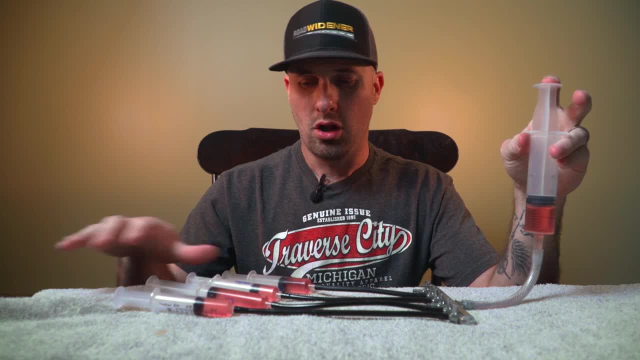 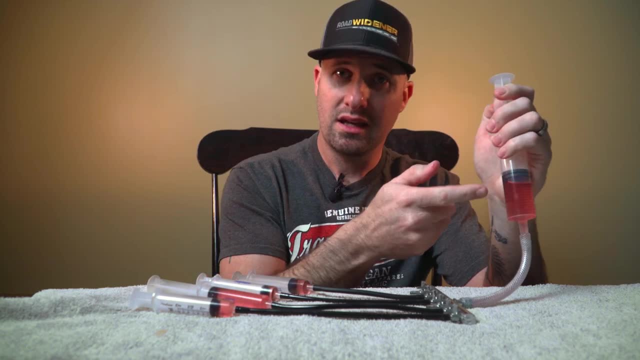 simple hydraulic system to where now I can make all of the cylinders go out at the same time. And again, in a real world we would not retract them like I am now by sucking the oil back in. We would actually pump oil to the back side of this. 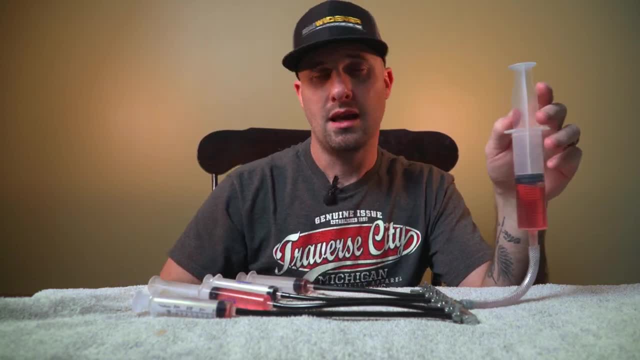 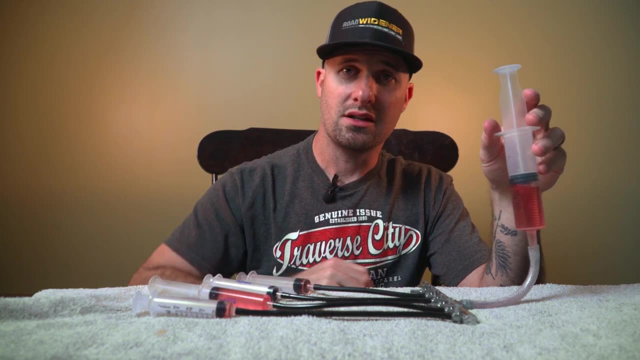 piston here and it would drive the cylinder in And, by the way, there is a valve that opens and dumps that oil back into our hydraulic reservoir here. So it's a complete circular system. it's a complete closed system. So what we can do is we can have all of our cylinders working at the same. 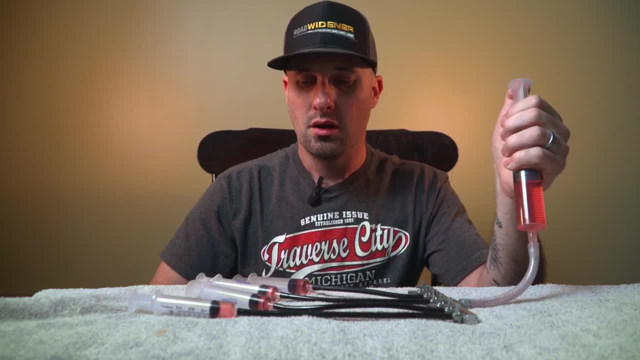 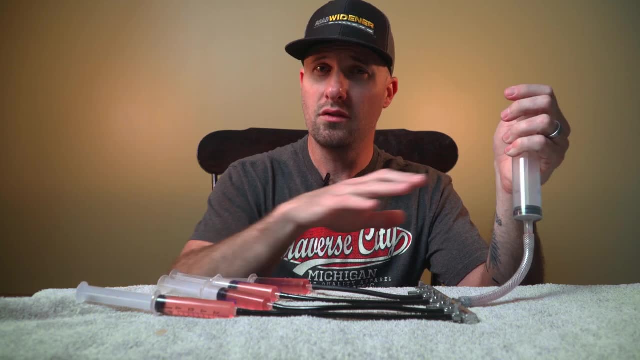 time with all of our valves open. One thing I want you to note: I'm using a lot of hydraulic oil, I'm using a lot of force, but look at how little all of my cylinders are moving because all of this fluid that's running through this line here. 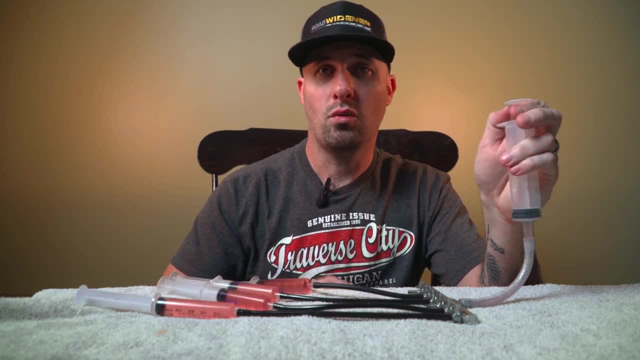 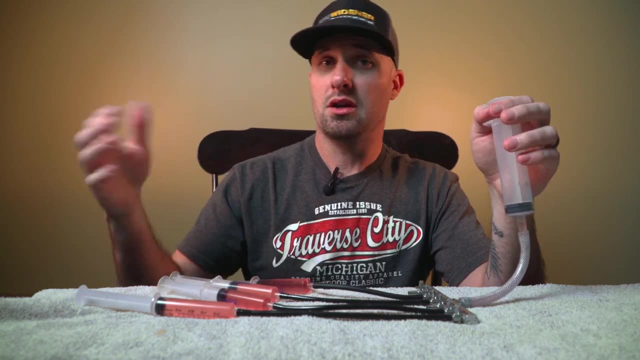 Can split between four separate cylinders. That's why, when you do multiple movements, especially in an excavator, when you're curling your bucket, you're sticking in, you're booming up and you're turning all at the same time. it doesn't work as fast as it does when you're just sticking in and 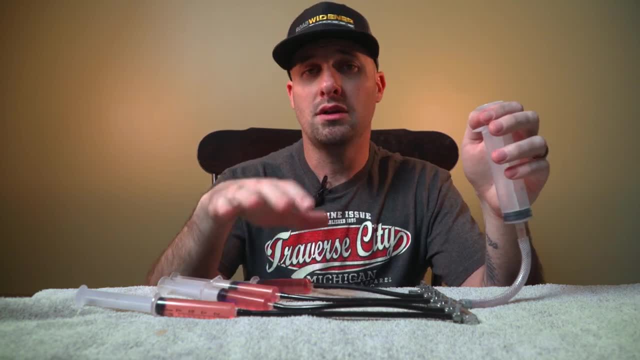 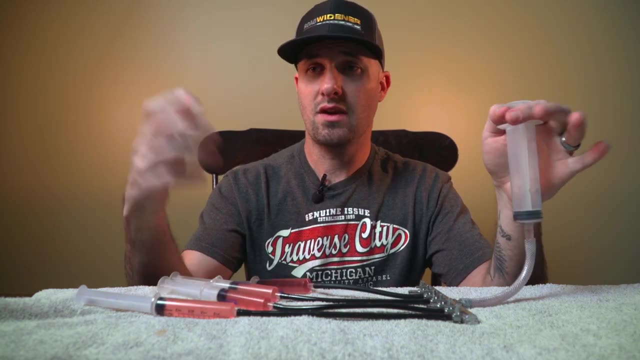 turning, or when you're just turning, And it's because the pump can only output so much hydraulic oil at a time. And if you're splitting that between four or five, six functions, you know, let's say you've got a hammer on there too that's running at the same time you're doing. 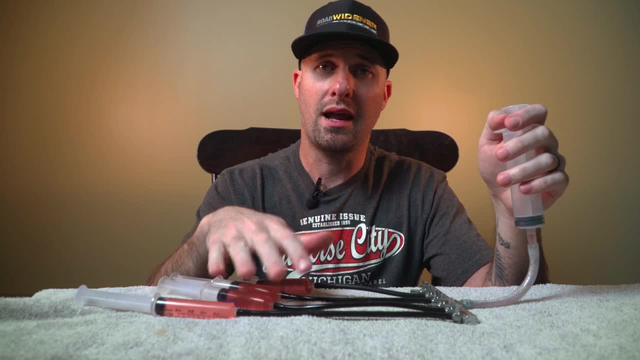 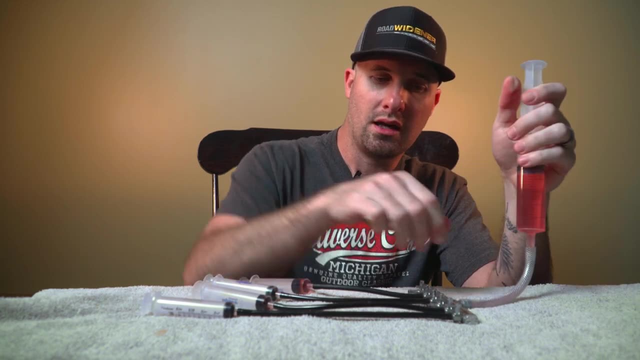 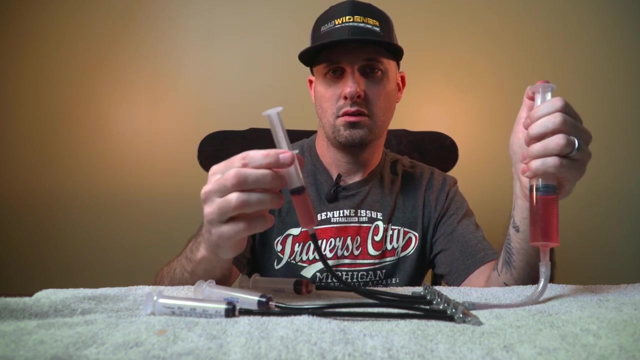 everything, it's all going to slow down a little bit because you're limited on how much oil can actually run through the system. So the way you get around this is: let's suck our hydraulic oil back in here. If we close a couple of these valves now, I can work this one cylinder with very little. 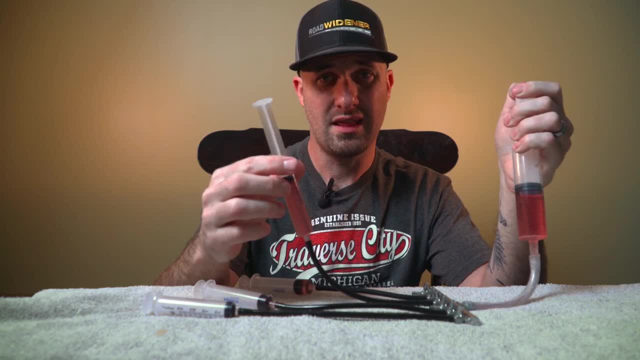 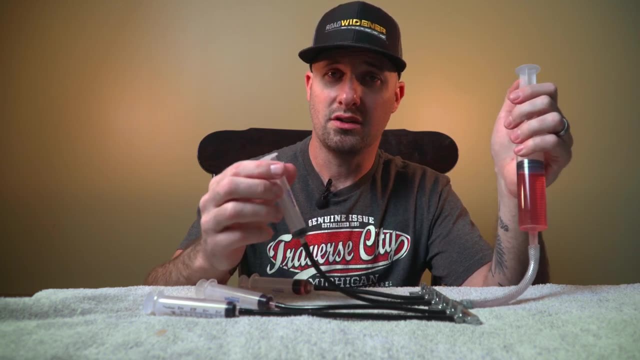 effort on my pumps part, So you can see that my pump is not moving that much, but we're getting a lot of action out here on our cylinder. So that's how you can move faster in an excavator, and efficiency is by trying to limit the number of functions that you're doing at one given time. 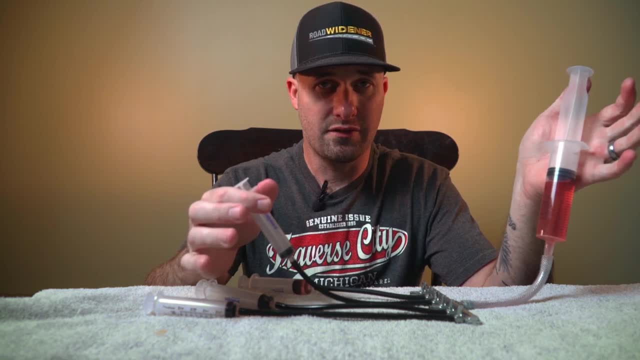 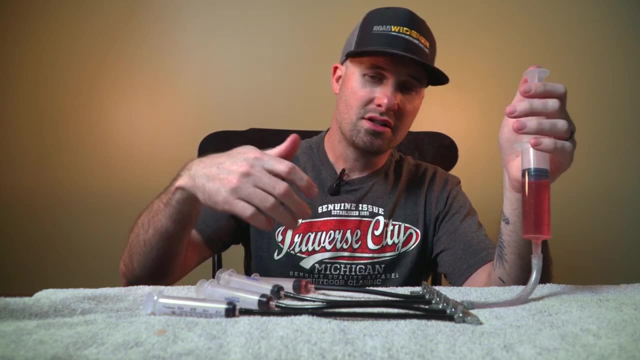 Now, obviously you have to do certain functions at the same time in an excavator to make it dig. But, like I talked about in my tips and tricks video, if you're turning back over your pile and you're sticking out and you're putting your bucket, you know uncurling your bucket and you're booming. 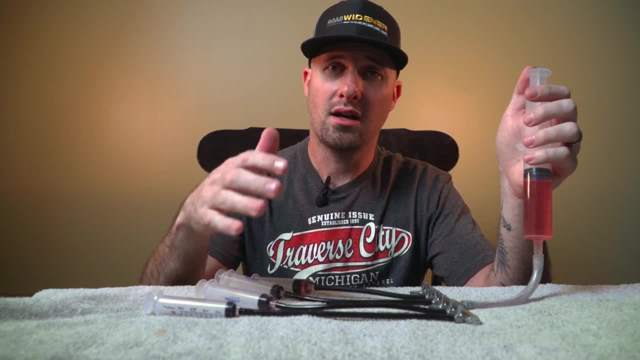 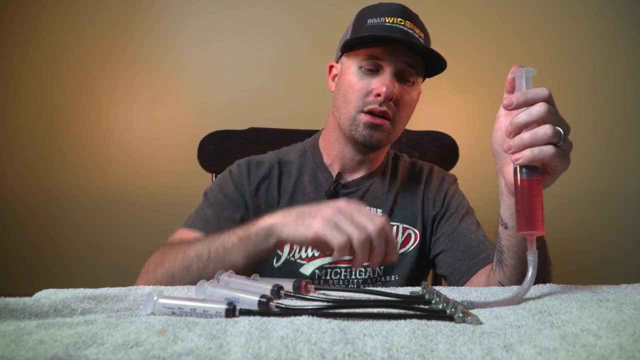 down all at the same time. it's going to slow you down And that's why I talk so much about wasted movements is because of this concept. right here, You only have so much flow that can go through the system, So we could open another valve and we're only working two cylinders. It's going to slow down. 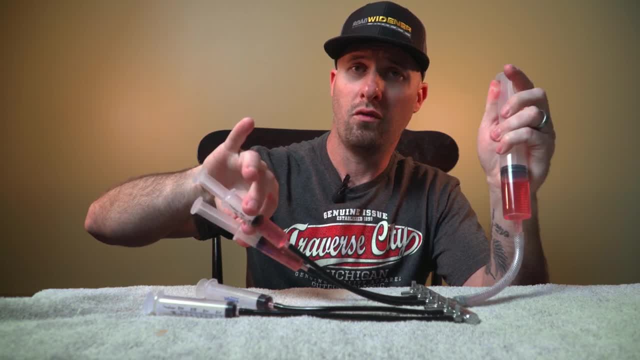 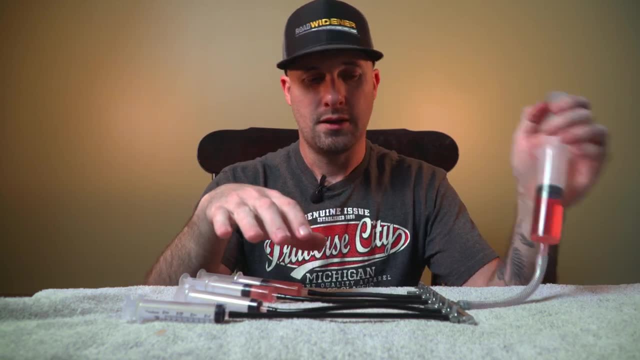 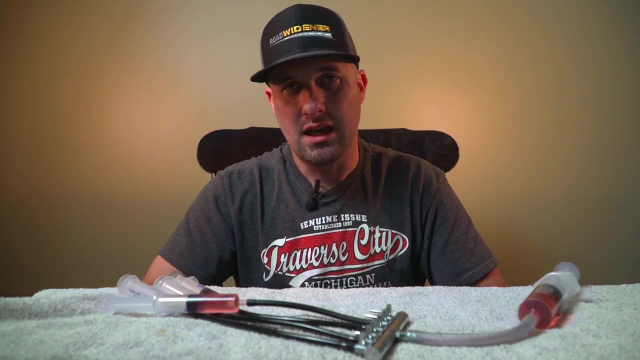 a little bit, but still we're a lot more efficient than we were by opening all four valves. So another important concept here is limiting the amount of oil that you need, And this is why, in all honesty, this is why- hybrid machines in the market are going to be such a game changer. I'm 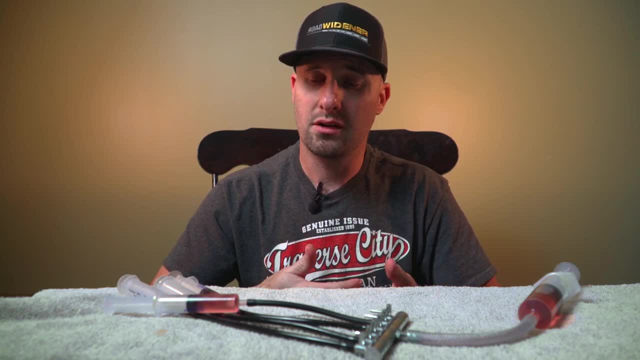 going to speak about Cabelco excavators just because I used to sell them and I know more about those than the other manufacturers. But there are a lot of other machines out there that are going to be able to do that, So I'm going. to speak about Cabelco excavators just because I used to sell them and I know more about those than the other manufacturers. So I'm going to speak about Cabelco excavators just because I used to sell them and I know more about other manufacturers. 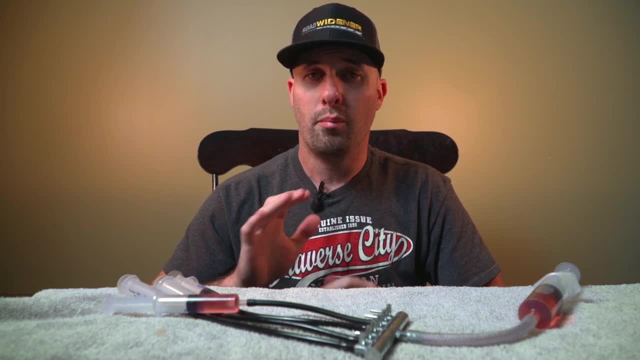 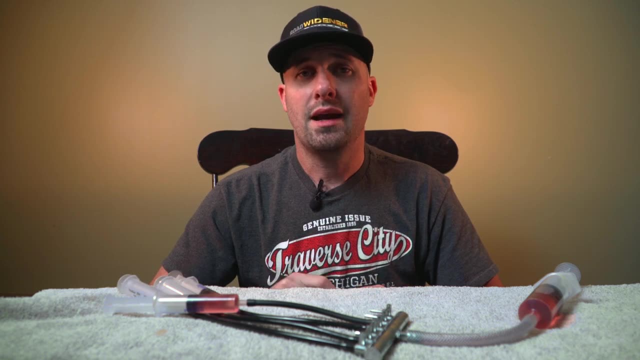 So I'm going to speak about Cabelco excavators just because I used to sell them and I know more about other manufacturers on the market that are coming out with hybrid machines. But the way Cabelco's machine works is your swing motors are no longer hydraulically driven, They're driven by an. 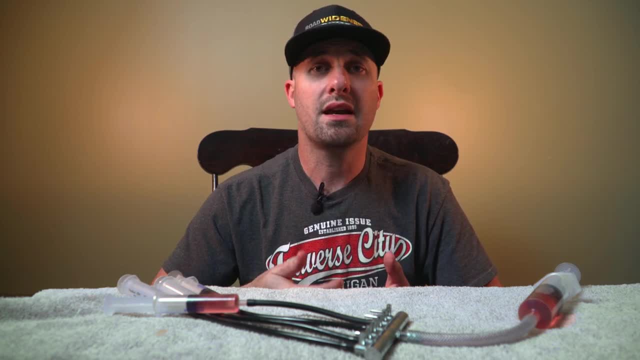 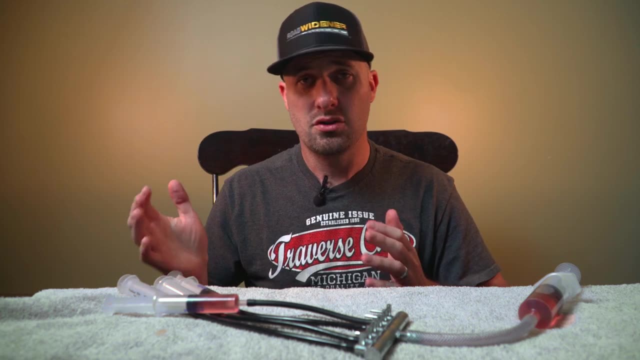 electric motor. So what does that mean? Well, swing motors take a lot of hydraulic oil. You're going to notice that, of all of the functions that you're performing at the same time on an excavator, as soon as you start to swing that machine, it really slows your hydraulics out on. 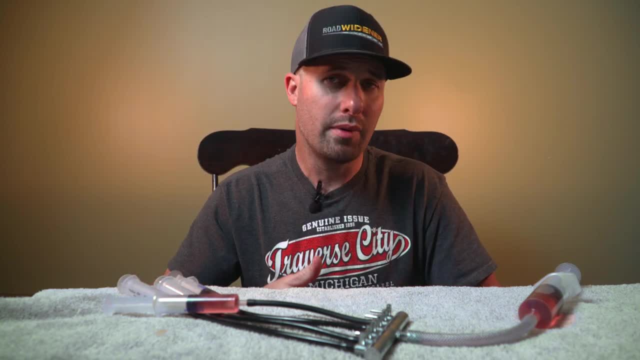 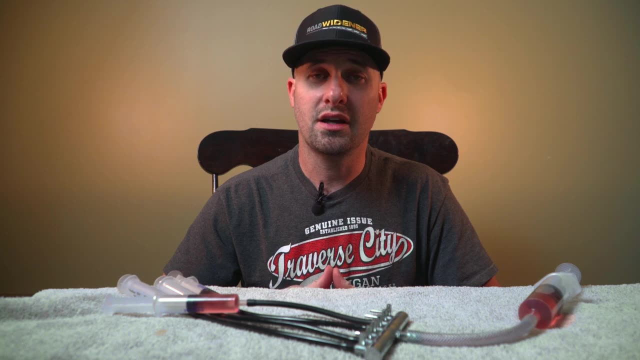 the boom and the stick and your bucket. It slows those way down. So, on a Cabelco machine, on a hybrid machine, the swing drives are now electric. Now we don't have a hydraulic circuit going to your swing motors, which means that we can swing at full speed while we are also sticking. 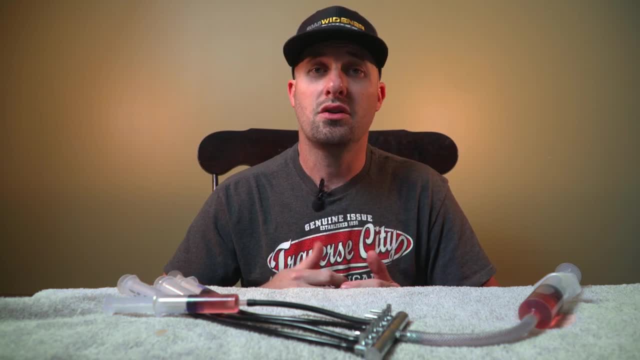 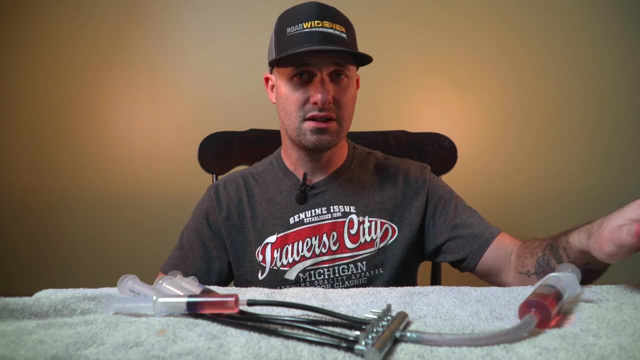 in booming up and curling our bucket at full speed. So you can see right there, take the fuel efficiency out when it comes to these new hybrid machines. Take the fuel savings out of the equation. Just from a production standpoint, that is a huge game changer on how many more loads you. 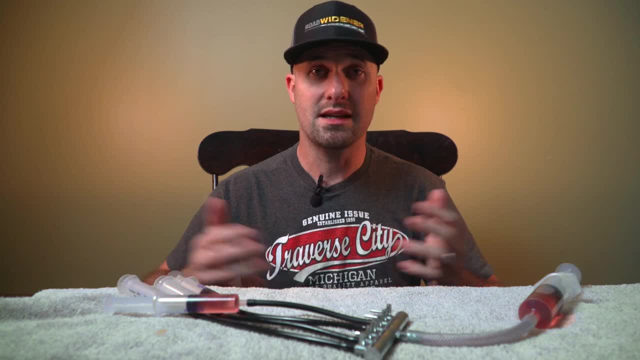 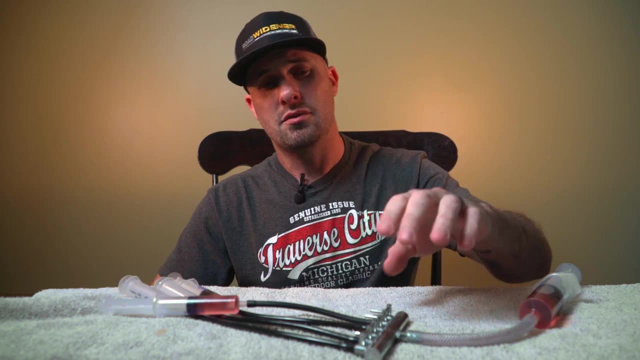 can put in your machine, So you can see right there. take the fuel efficiency out when it comes out in a day, because you aren't losing that time, that cycle time, bogging your hydraulics down with your swing motors. So that's another important concept to realize, Another concept to 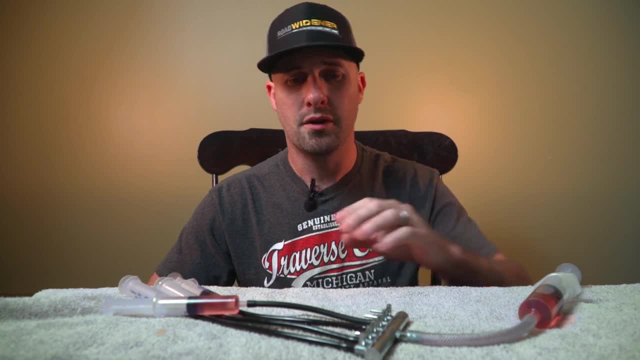 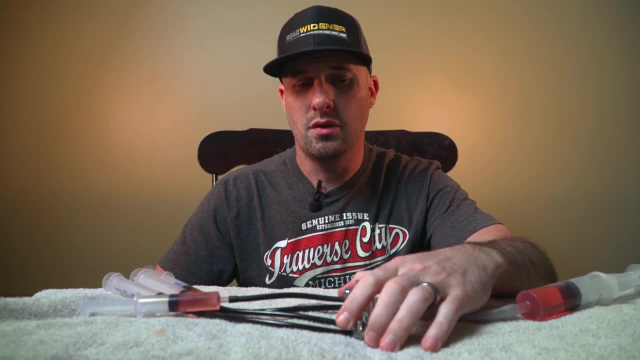 realize, or at least so that you guys understand these systems a little bit better, these valves I'm manually turning myself In any machine. these valves are generally controlled one of two ways You may hear of a pilot system. So when you hear of a backhoe or something along those lines being 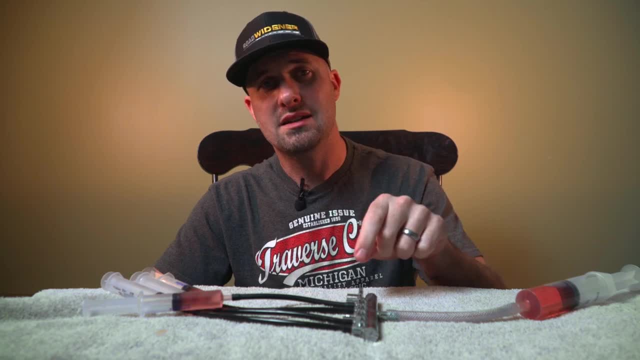 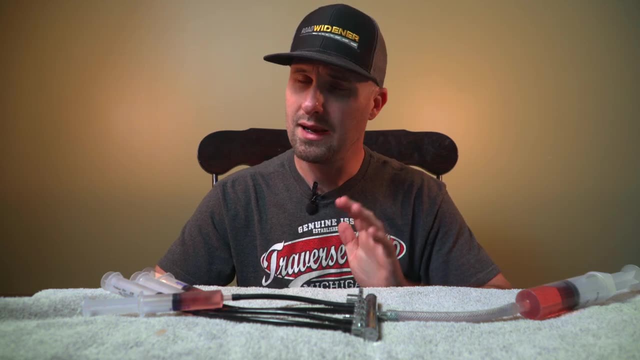 pilot controls. that is where you actually have to be very careful. You have to be very careful that you actually have a second, smaller hydraulic system. It still pulls from your regular hydraulic oil, I believe. Don't quote me, I'm not a hydraulics expert- but I believe it still pulls from the same. 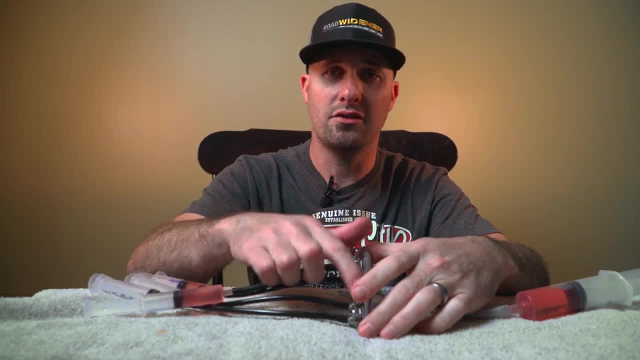 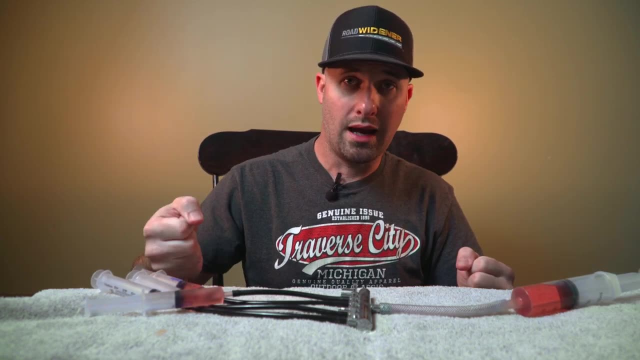 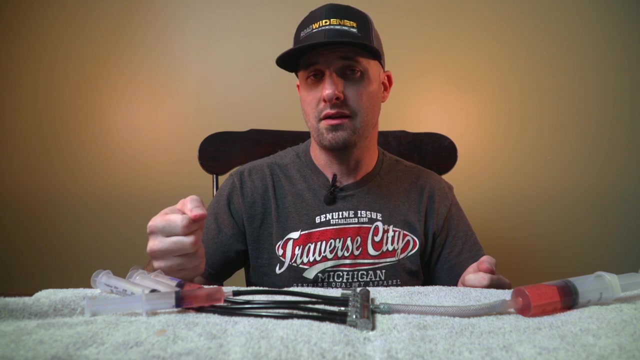 reservoir and everything. But you actually have a smaller set of hydraulics that control these valves And that system is tied to your joysticks and the cab. So when I push forward and I boom down on my skid steer or on my excavator or whatever I'm driving, I actually have a hydraulic. 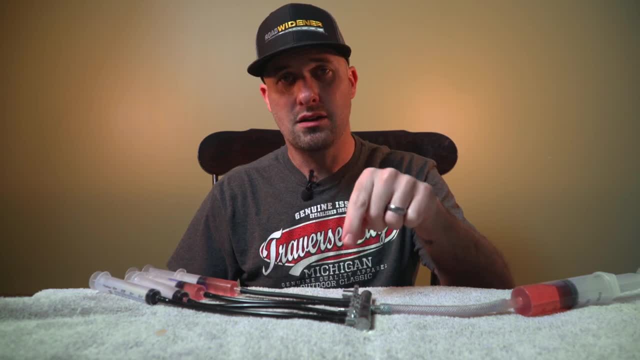 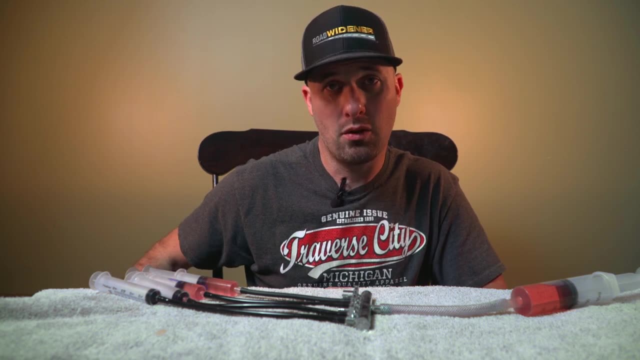 system that controls these valves And that system is tied to your joysticks and the cab. So when I line, that is going to this valve and it is mechanically opening this valve. That's why pilot controls actually generate a little heat in the cab If you put your hand down where 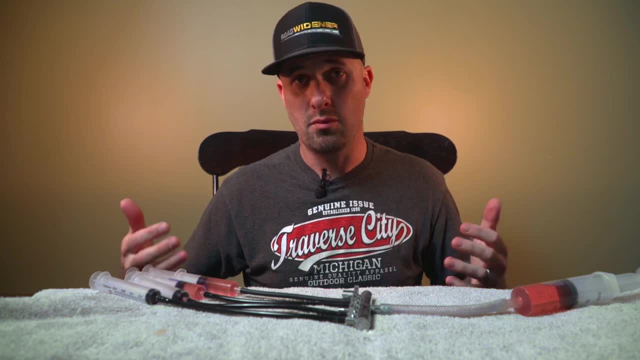 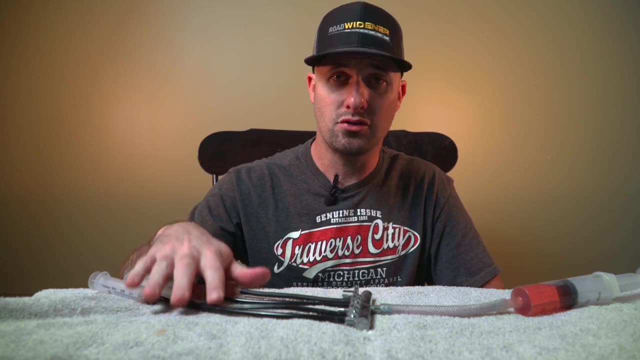 your controls come out of the console or out of your armrests, you'll actually feel in a pilot control system. there's some heat there, and it's heat from the hydraulic system. There's actually hydraulic oil in the cab with you, So that's how a hydraulic system works with pilot controls. 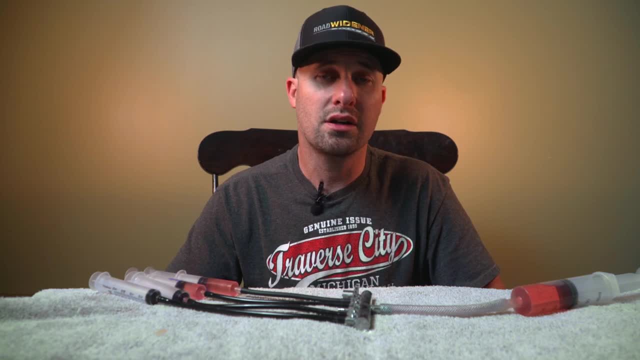 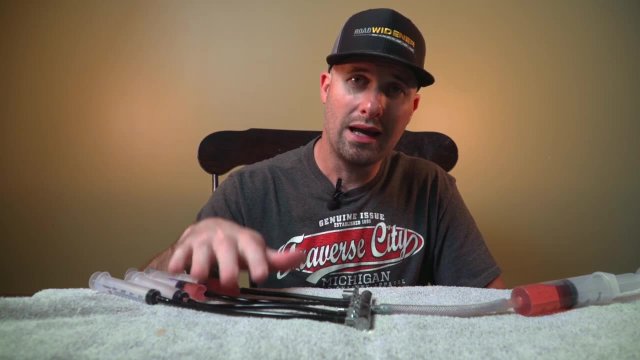 The newer style of controls that most guys getting into the industry are going to be used to are actually what they call EH controls, or electronics over hydraulics. Instead of having a pilot control system that's going into the cab, all of your joysticks have sensors in them. 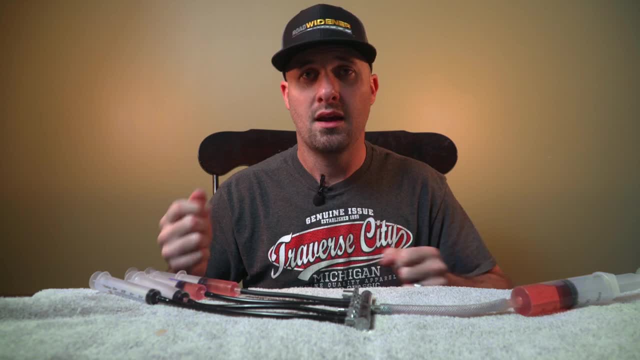 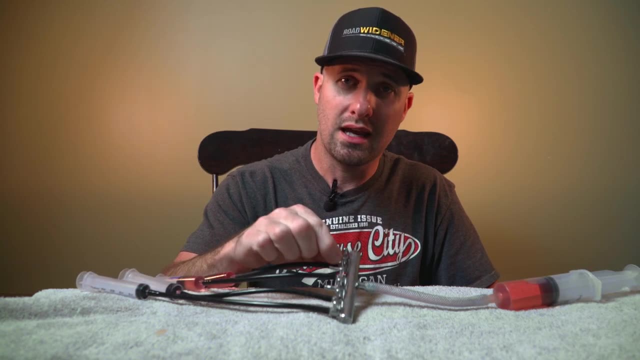 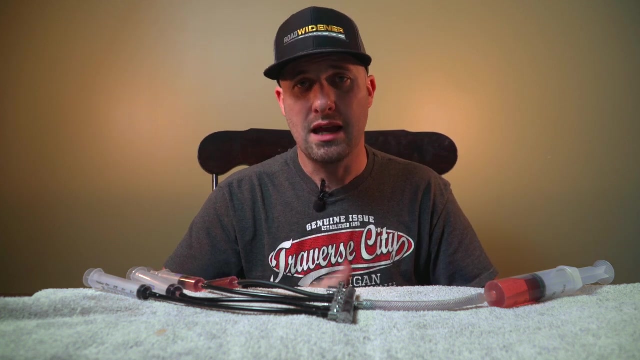 that detect how far you're pushing the joystick. That electronically communicates to a solenoid, which is just a fancy word for an electronic valve. It communicates to a solenoid and it opens the valve however much the computer deems it. And that's why in EH controls you can actually go in and adjust sensitivities, You can change. 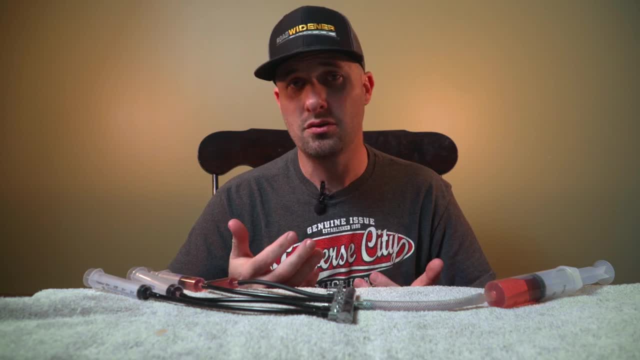 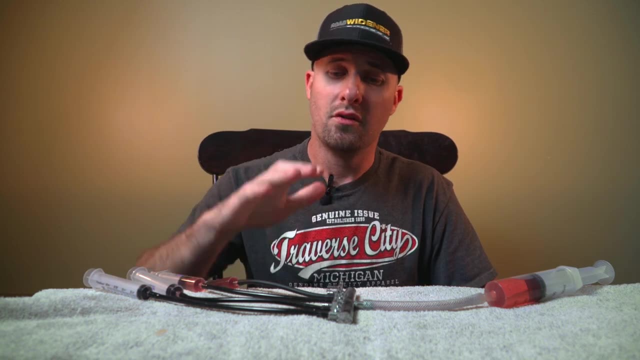 how quick the valves respond to what your inputs are. You can't do that on a pilot control system. It's all in how much you are allowing hydraulic oil to move through that system versus EH. You can use the computer and actually dial that down. So there are some drawbacks to that system With. 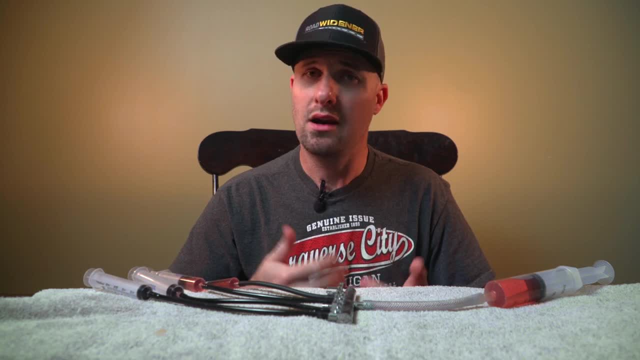 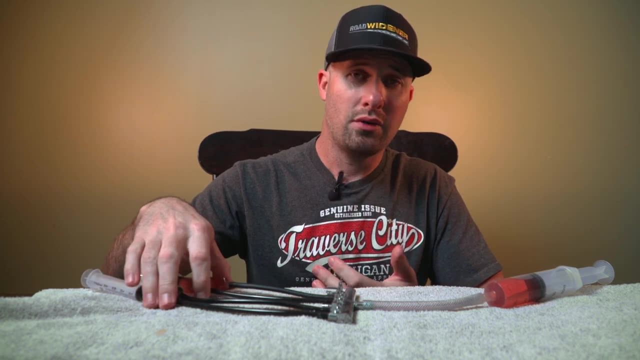 an EH system, you lose the feel in the controls And a lot of old school operators are really used to great control systems And a lot of old school operators are really used to great control systems Grading with the feel in the controls themselves. When I ran loader for a long time, I originally 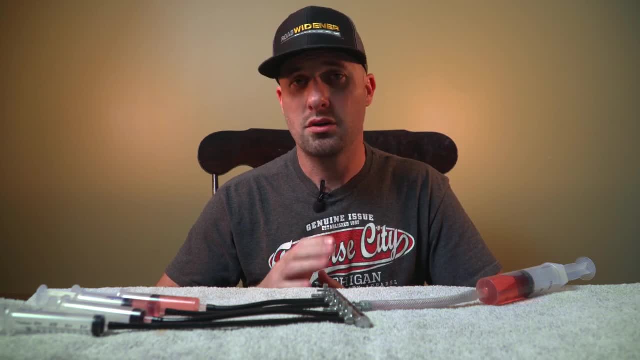 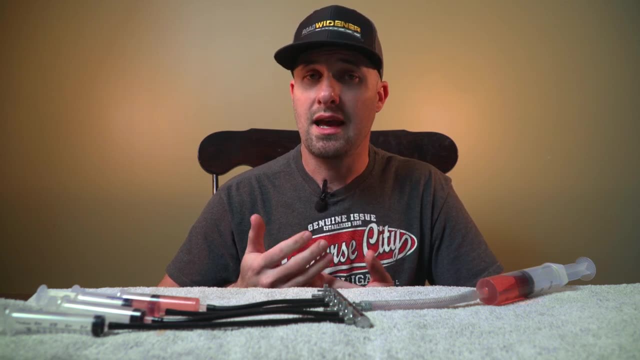 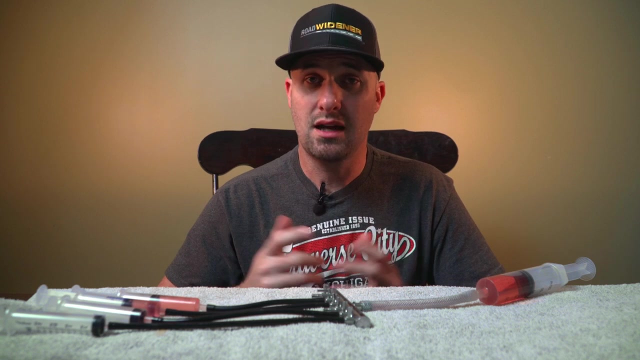 started in a pilot control system and I 100% graded by feel in my controls When I switched over to the CAT 938, it was a K-series that had EH controls, Believe it or not. I had been running loader for about a year and a half at that point And I had it down pat. I was a decent operator in. 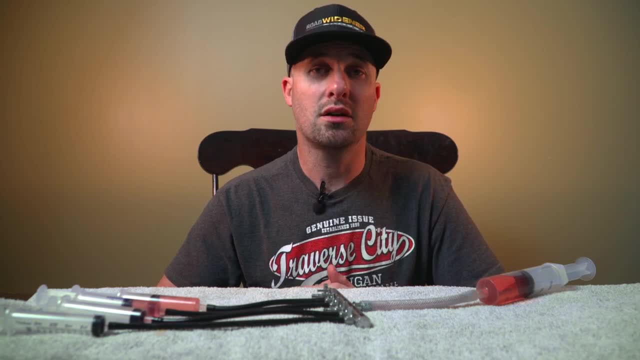 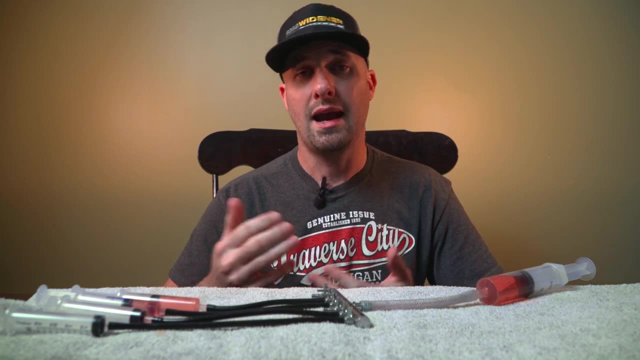 the loader. I totally. it took me about four days to totally relearn how to grade in that machine. I no longer had the feel of where that bucket was level and contacting the ground. I had to learn how to get that from my seat, And so it's still doable. You can absolutely learn to grade in one of the new 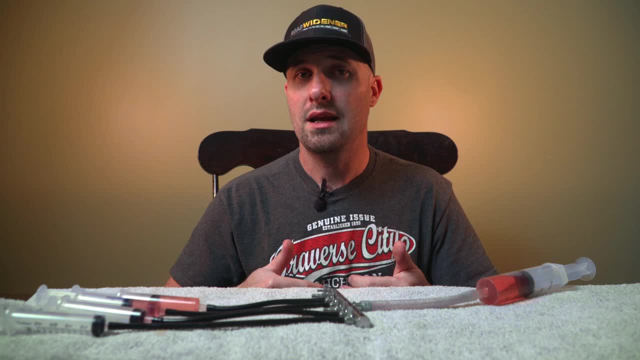 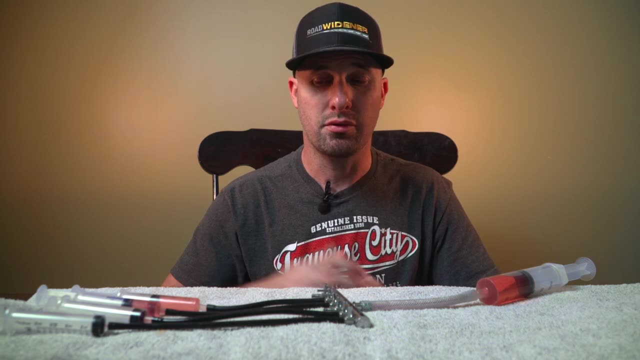 age machines. You're just learning a different way to feel the machine and what you're doing, and when you have resistance You're no longer getting that feedback in your hands, like most operators are used to. So that's another system. The third system: that's not nearly as common, it's generally. 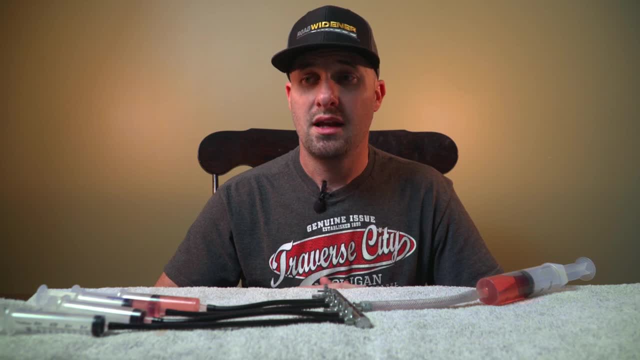 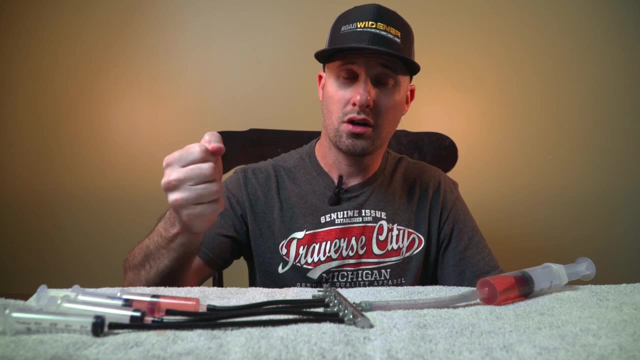 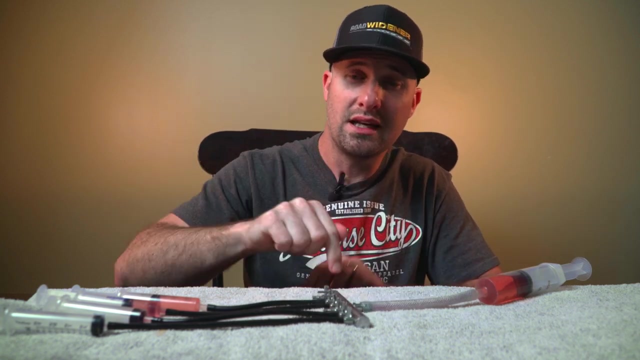 reserved for smaller skid steers And stuff like that is a mechanical valve system And that is actually. you have a linkage that hooks your control arm down to this valve And so when you push forward, you're physically causing the linkage to lift that up so that that valve can open and allow hydraulic fluid through the system.